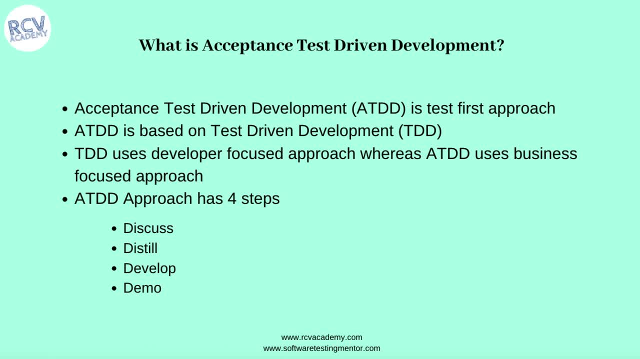 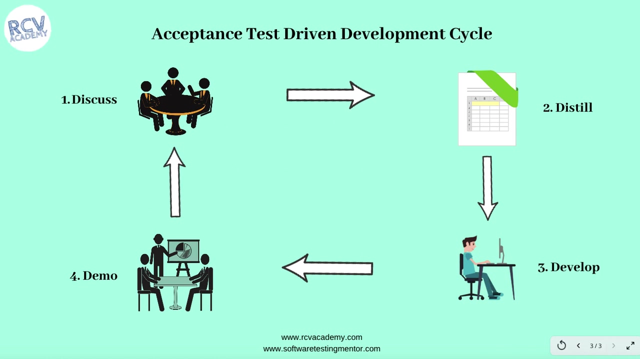 wherein you first discuss within the team, Then you still what are the criteria? didn't develop and demo. so let's see what are these four approaches and what all steps or key work items are involved in these four steps. so let's go ahead and see what is involved in the discuss approach, so discuss in the discuss step. this is the first step. 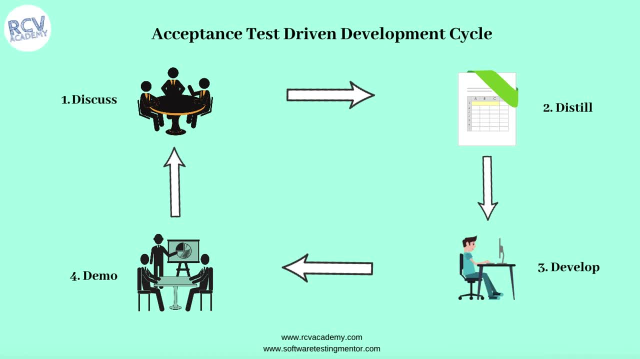 of the workshop and in the discussion step you discuss the user story or the work item. that needs to be done with the whole team, so it's analyzed, it's discussed and by within the developer, tester and business stakeholders to come up with any ambiguities or in an incompleteness or errors in the user stories. 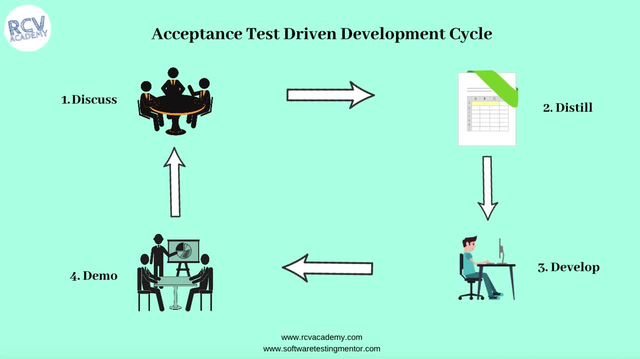 and then, once everyone in the team is happy and all the open questions happen been identified in the discussion and addressed, the next phase of of that user story is to distill that user story. and when the discussion is finalized and user story is finalized, the next step is to distill that user story. in distill, 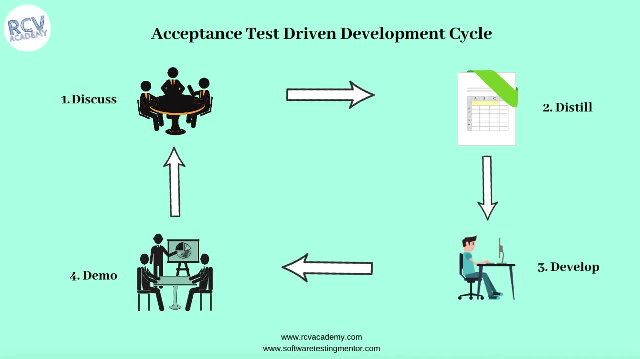 step it can be done by the tester only. like in first step, you have the developer development team, you have business stakeholders involved. however, in the next step, which is a distal step, there could be the development team involved or only testing team doing the distal work of the user story that has. 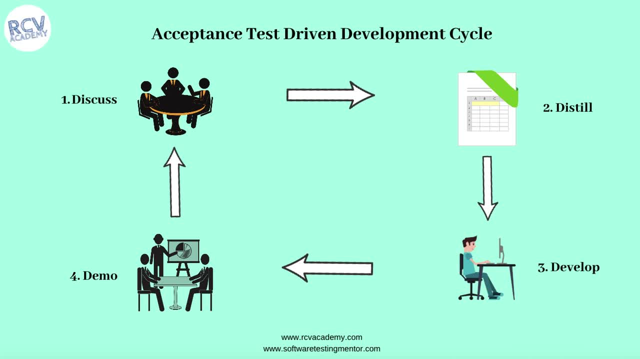 been discussed and finalized in the step one, what is done in the distal step? tester writes the scenarios or the test cases or acceptance tests based on the test cases or acceptance tests based on the test cases or acceptance tests based on the acceptance criteria defined in the user story. so he has been involved in the 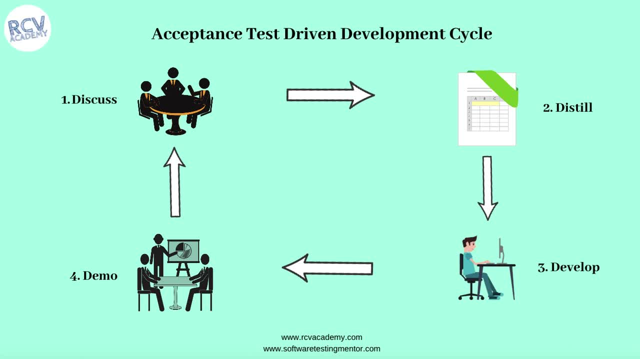 acceptance criteria defined in the user story. so he has been involved in the discussion step already. he knows what all acceptance criterias have been defined for that particular user stories. based on those acceptance criterias he'll come up with the acceptance test scenarios in the distal step and those 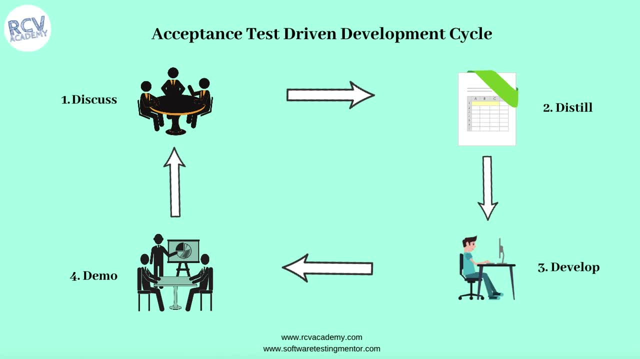 acceptance test. test case scenarios are then documented by the tester or they are documented by the test case scenario, so standing answer is deliverable automatically. the test case scenario is done for all acceptance criteria. there might be possibility that even more people, or even the developer, is also involved in. 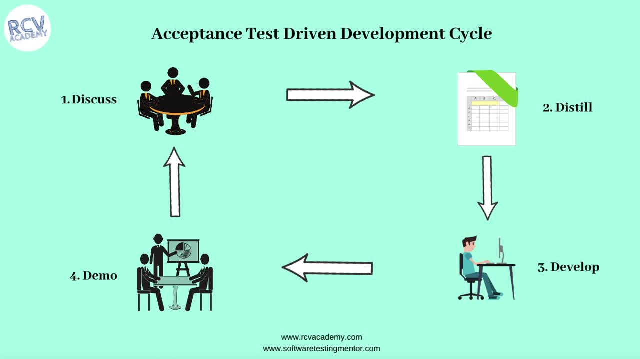 the distal step just to get more perspective of different people within the team. once these test cases are defined, then the next step is to come up all the positive conditions that confirm the acceptance criteria defined in the user story. the next step is to also come up with the scenarios or the negative scenarios that might be. 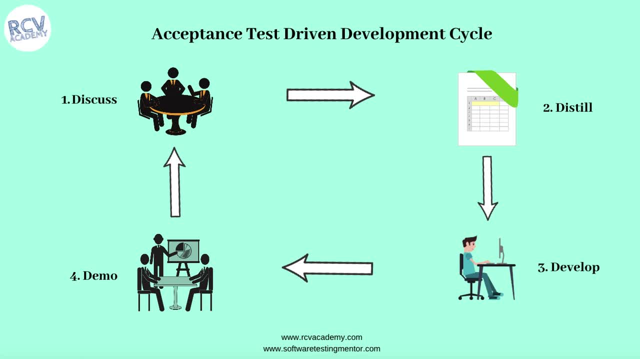 required to be addressed for that particular story. apart from negative scenarios, you could all you also need to come up with the functional security and any other different non-functional attributes of that particular user story. so that's all. uh, what happens in the distill step? once all the 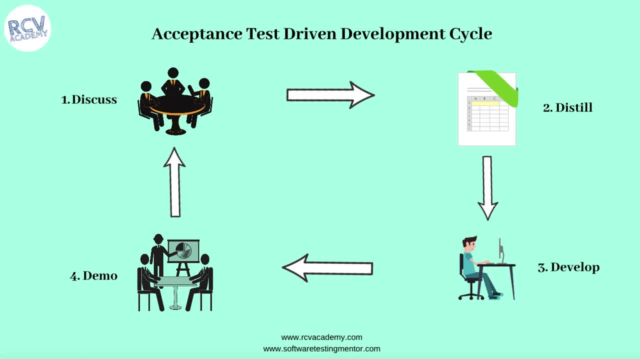 positive scenarios, negative scenarios or non-functional aspects are being defined in terms of acceptance test cases. then the third phase is the development phase. so now you have the set of complete user story, which has been discussed in first step. any ambiguities have been addressed. next step has been completed. 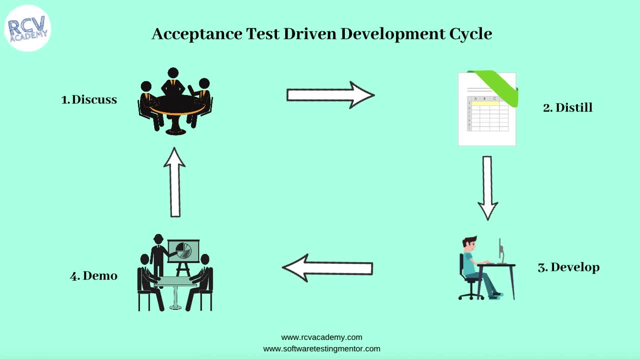 which is the distal step, when the the tester has documented all the acceptance test cases. the third step is to start developing the user story, or to do the actual coding, wherein now the developer starts writing the code in similar to test driven development, but however, he just 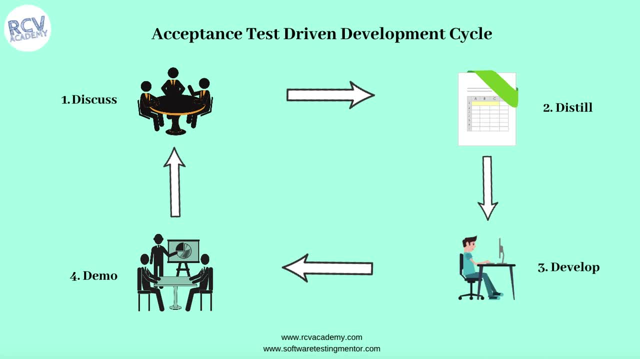 refers to the acceptance test cases written in the step two, which is the distal step to meet the acceptance criteria, or the test cases that have been documented in the step two. now, once the coding has been done and all the acceptance test cases that have been have been.